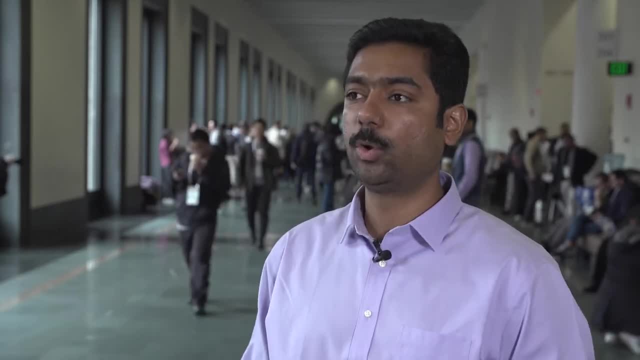 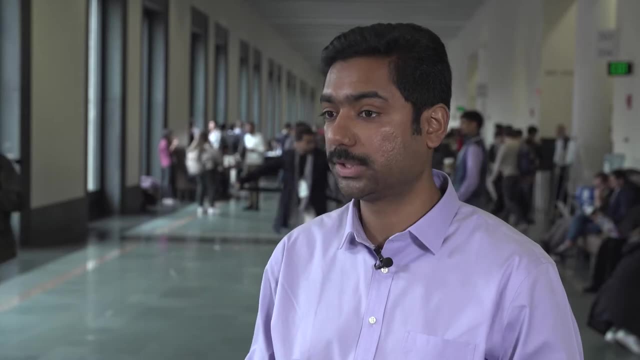 test different materials, you know, until you find success is no longer the best way to go. So it is widely accepted that you know these. these ML, data science, AI related approaches are seriously the future, are the way to go. Autonomous experiments are the future and they are built on machine. 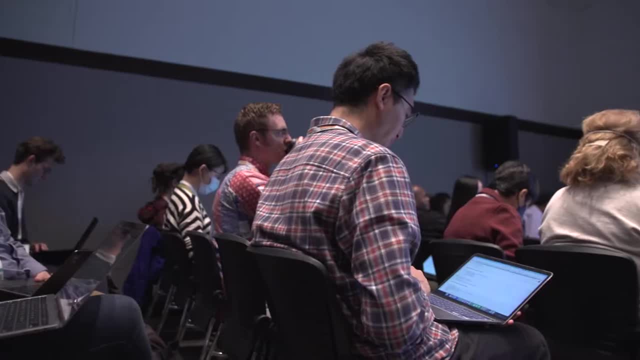 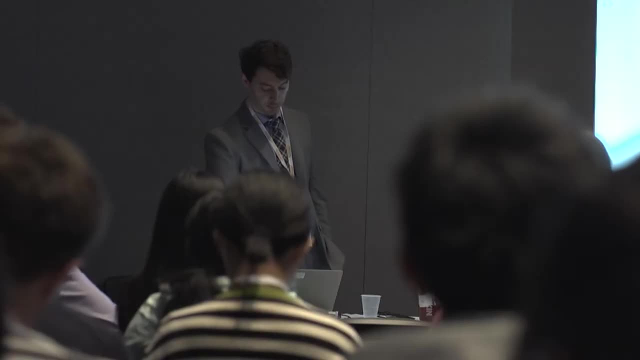 learning and data science. Now that's where this tutorial comes in. So we realize that you know, a lot of people are using machine learning in material science, but a lot of people are still not. A lot of people, especially students, you know. beginner students do not. 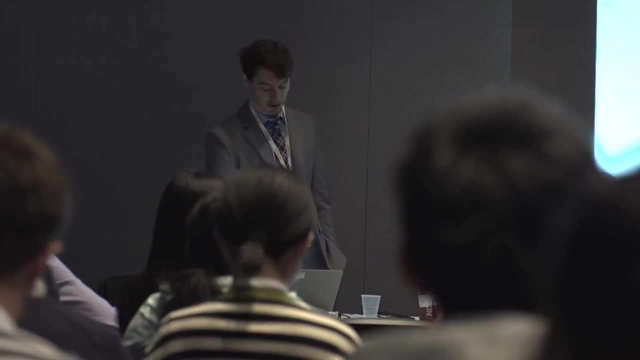 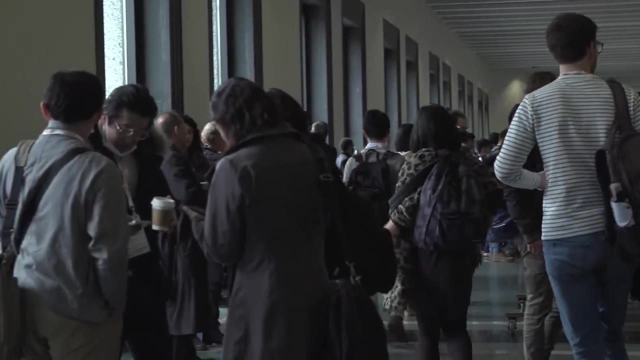 quite know. you know what it is like and how easy it is to pick it up, especially So what we're trying to do with this tutorial is to give people a basic introduction. Here are the essential concepts. Here is what you need to know, like the nuts and bolts. okay, It's very simple. you don't? 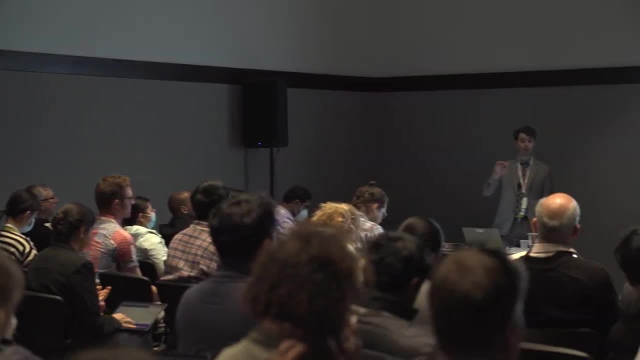 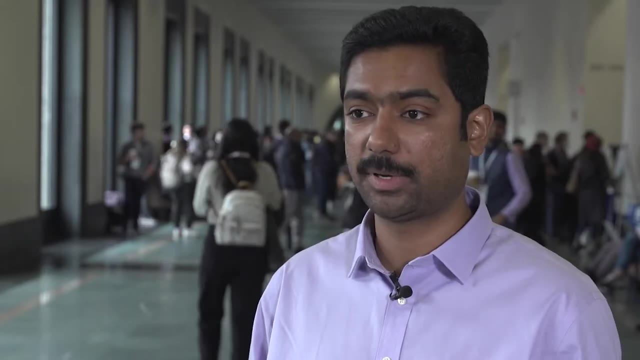 need to know all the theory behind it. Take these codes, take these scripts, take these notebooks that we have. apply it to your data set. Here are the basic concepts behind it. So anybody, any experimentalist, any computer scientist, any computer scientist, any computer scientist any. 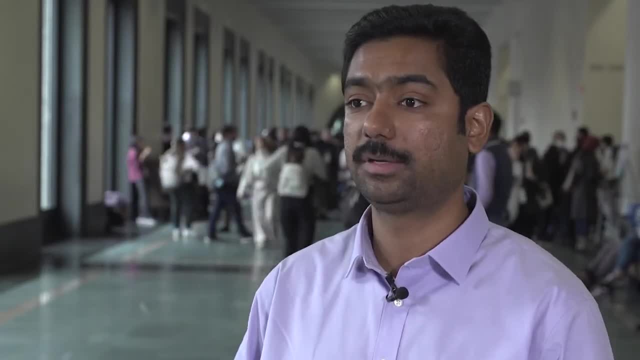 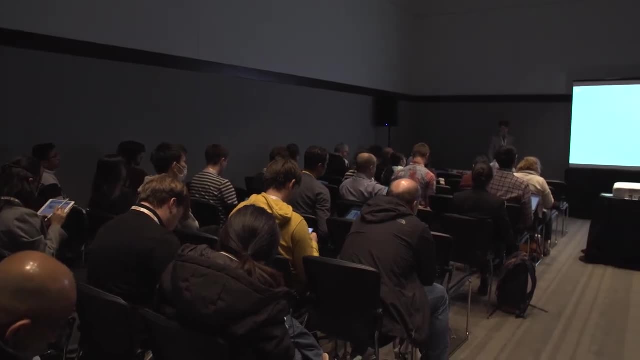 computational person, any material scientist, can now take it, start using it for their problem. So that is, that is the idea. So I cover essential concepts of you know what are the types of machine learning and the methods, specific methods like neural networks or other regression methods that 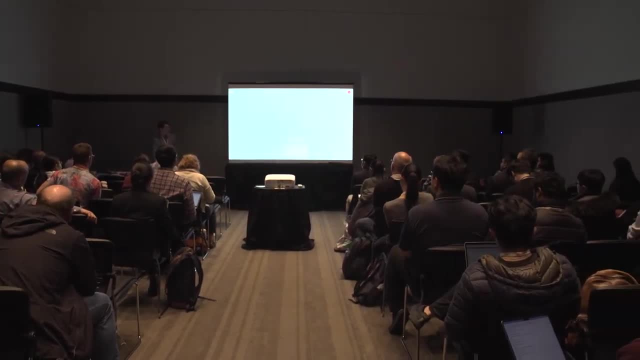 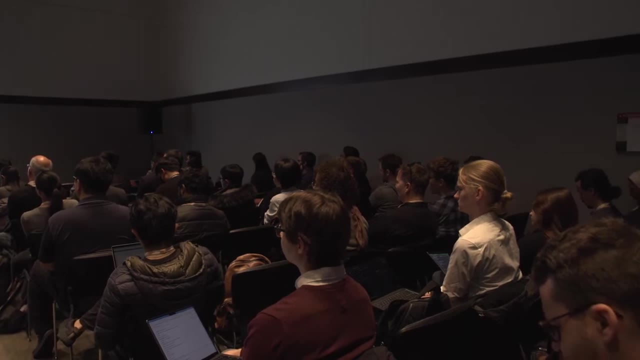 you may apply classification methods etc. And then I give a detailed example from my own research, which is on perovskites. So I present, I show people how you can visualize the data and how you can train simple regression models, how you can improve these models. Then 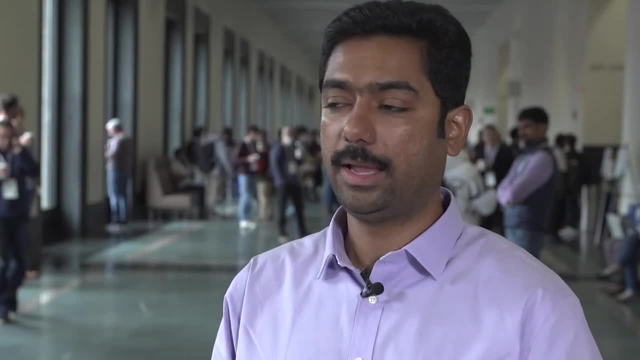 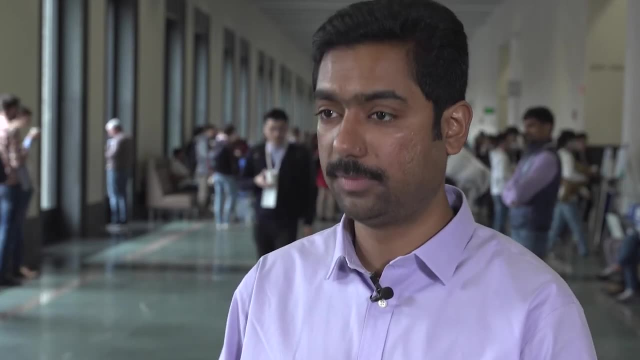 how you can use these models to discover new materials. In the next part of the tutorial we cover gaussian process regression, which is a specific type of regression method, and active learning. After that, we are going to cover neural networks in some detail. Neural networks are their. 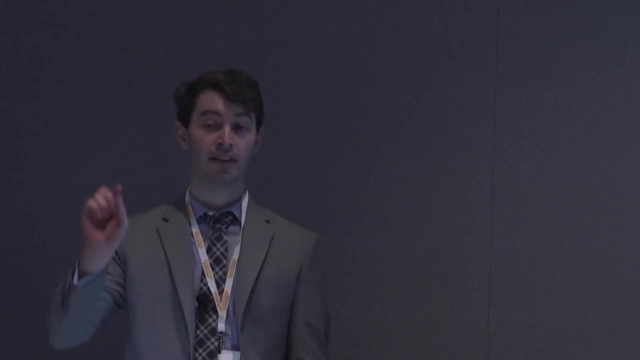 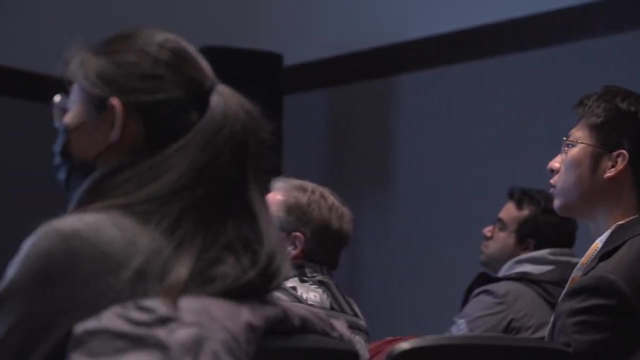 whole field. you know they are neural networks are used everywhere, like self-driving cars are using some sort of neural networks, for example. So it's a it's really a whole day where we are covering a few essential concepts that we think are the most important. It's a very exciting field, if you don't. 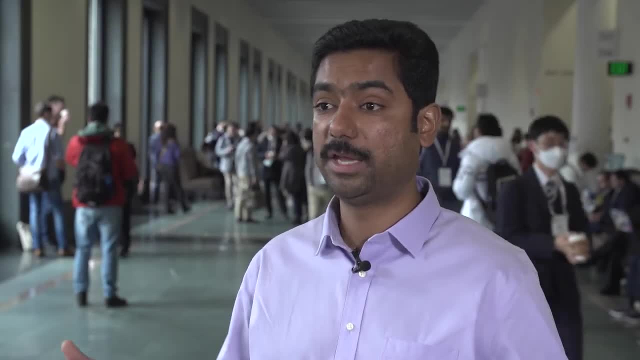 do machine learning, I encourage you to get into it. If you don't do machine learning, I encourage you to get into it. I encourage you to read many of these review papers that are out there and you know it's very interesting.